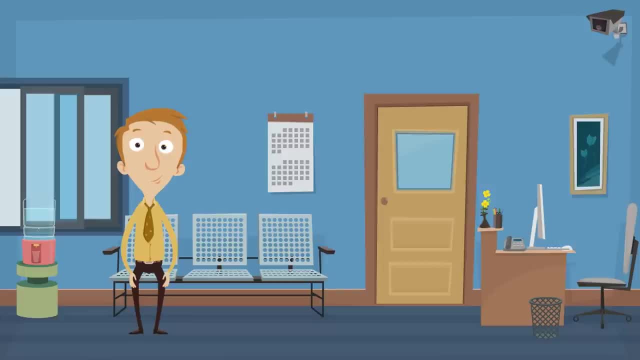 and it's a good time to think. You know, you can think about all kinds of things Like, okay, I have eight cowboy hats. I know it's crazy, it's weird: Eight cowboy hats and they're all the exact same, The exact same hat. I've got eight of them: Eight brown cowboy hats. 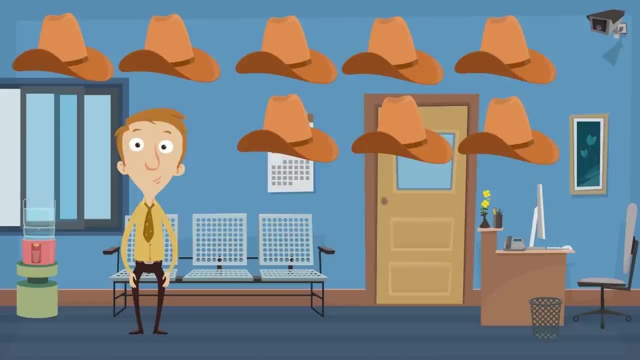 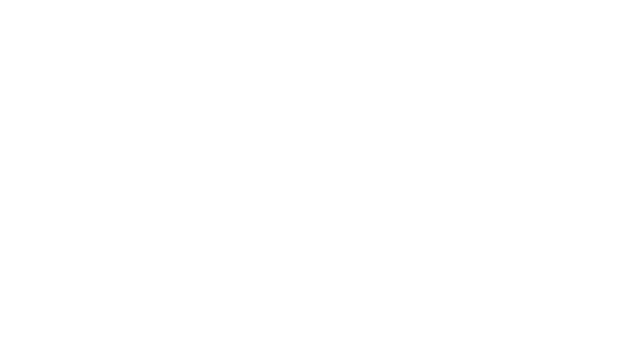 I mean, what's a guy going to do with eight brown cowboy hats that look the exact same? What could I possibly do with eight brown cowboy hats that are all the same? I mean, I should probably give some of them away. You know, I could give away one of my hats. 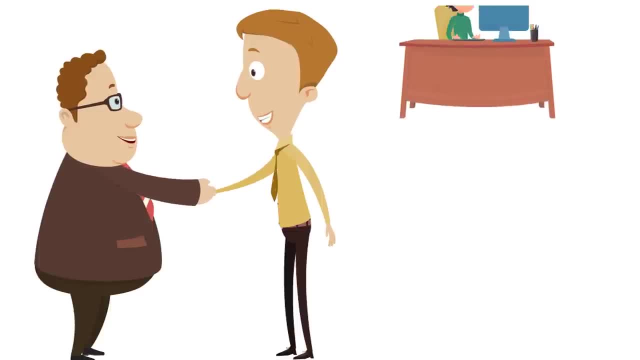 to Bob And Cookie might want one. Yeah, she might like a brown cowboy hat. you know I could give one to Nancy, you know, just in case she ever got invited to a western party And Chomsky he'd take a hat. 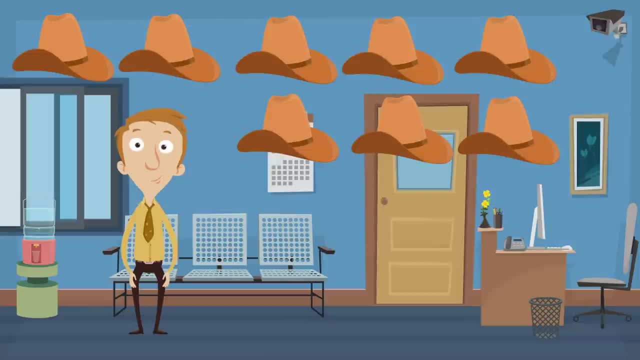 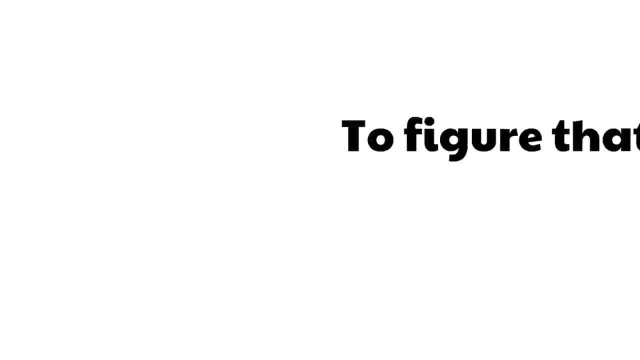 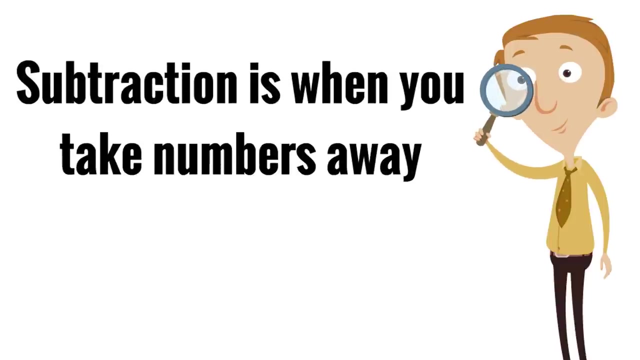 So, as I'm sitting here thinking about my eight hats, I need to figure out how many hats I'll have left if I give some of them away. To figure that out, we need to use subtraction. You see, subtraction is when you take numbers away. Yeah, very simple. Subtraction is when: 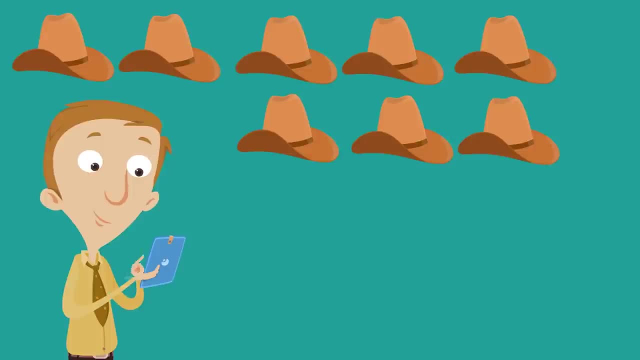 you take numbers away. So I begin with eight hats and I decide to give one away. We're going to need to subtract one from eight. The way we would write this is eight minus one. Now remember, when we subtract, we're just taking numbers away. 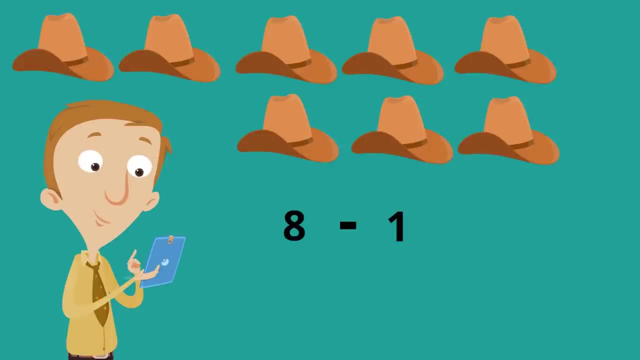 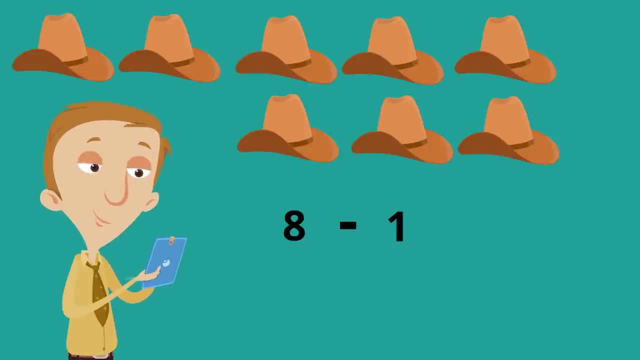 take one away. There we go. How many hats do I have left? What is eight minus one? If it helps, you can just count how many hats I have left. What is eight minus one? Yeah, seven, Eight minus one is seven. 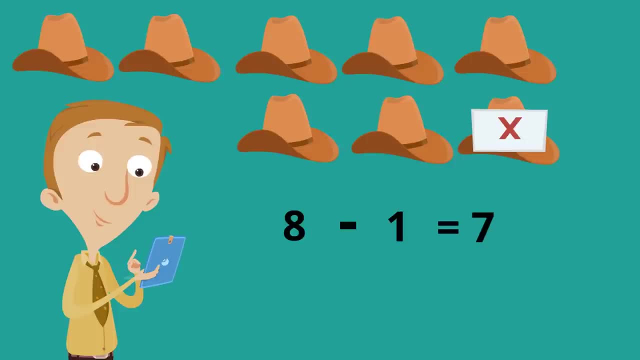 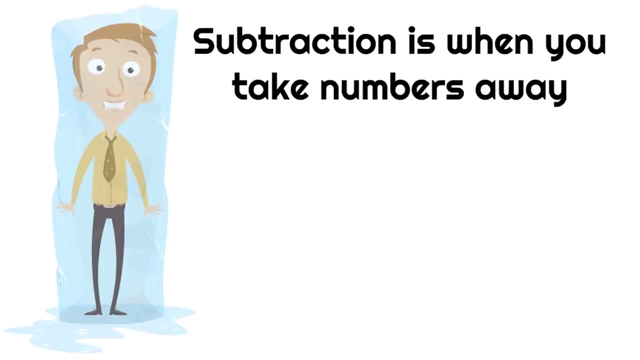 Now I have seven hats. Subtraction is when you subtract something away, Remember. subtraction is when you take numbers away And, as you might have noticed, we use the minus sign when we write a subtraction problem. You can see it right there in the middle. 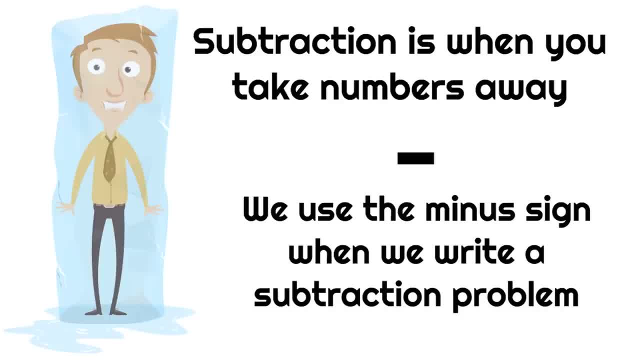 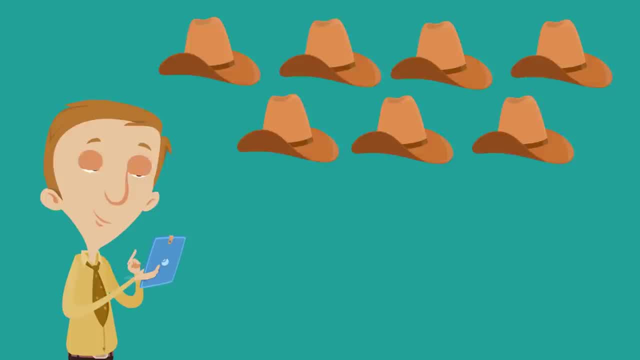 It's just like a dash. That's the minus sign. So now I have seven hats, but two of my friends stop by and I decide: you know what? I know, I just have seven hats now, but I want to give two of them away. 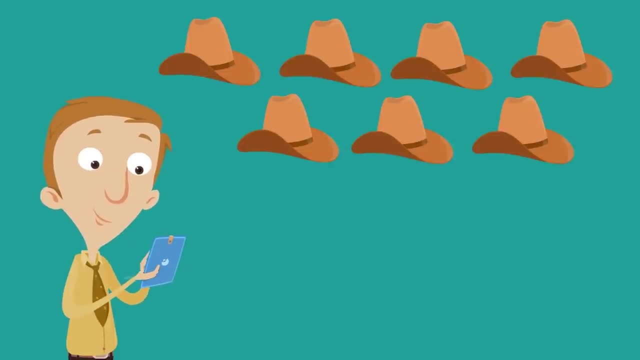 Now I'm going to be subtracting two hats from my collection. We would write this by saying seven minus two. Now let's take away two hats, We'll find out how many we have left. What a wonderful subtraction problem. What is seven minus two? 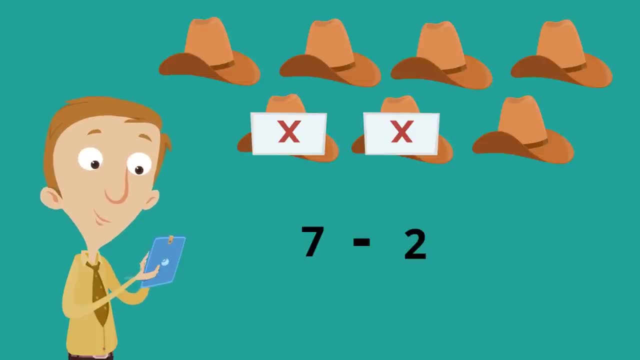 If you need help, you can just count how many hats are left. What is seven minus two? Seven minus two equals five. Yeah, Five hats, And you can even count them: one, two, three, four, five. There are five hats left. 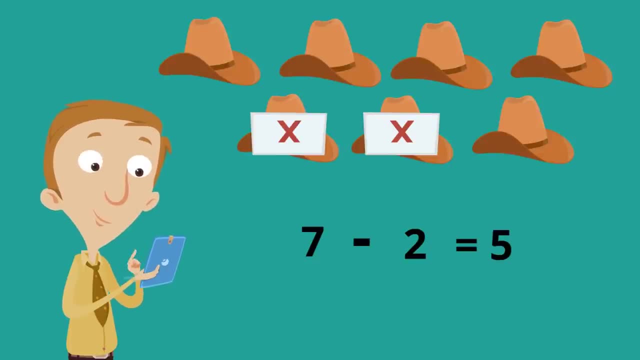 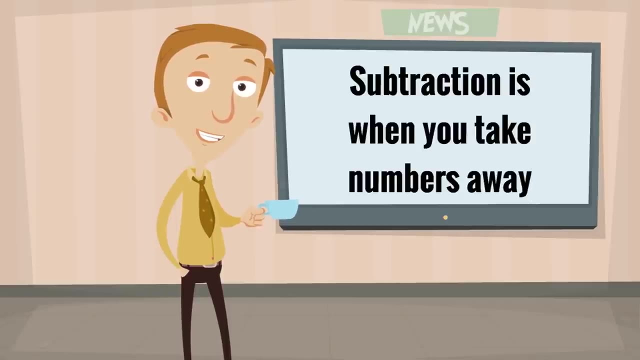 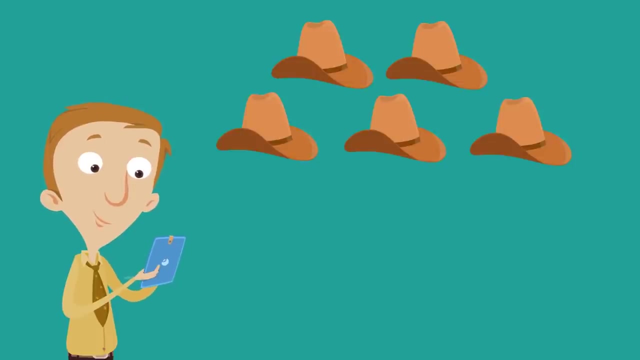 Seven minus two equals five. Do you see how fun and simple subtraction is? Subtraction is when you take numbers away. So now I have five hats, Five hats in my collection, Only five hats left. But then I meet up with my cousins Hooey, Dewey and Stewie, who want to have hats too. 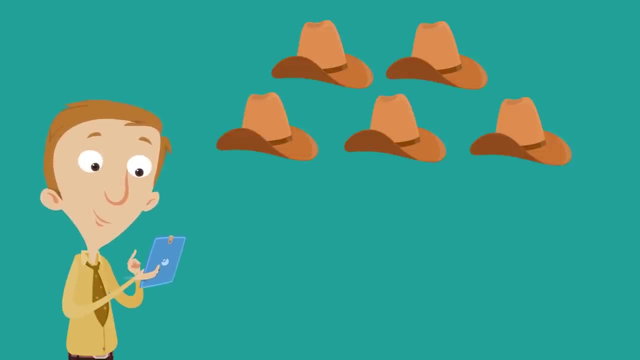 And I'd love to give them hats. So I'm going to give three more hats away. So I have five hats and we're going to subtract three hats. We would write that five minus three. Oh, I love subtraction so much, Oh. 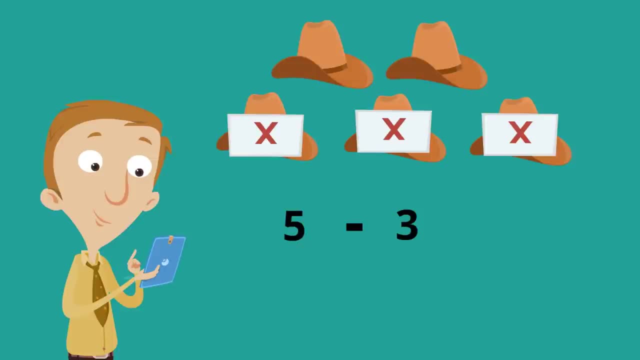 All right, Bada bing, There we go. The three hats are gone. So five minus three, how many hats are left? It's pretty simple, isn't it? Yeah, Five minus three equals two. Good job, Subtraction is just taking numbers away. 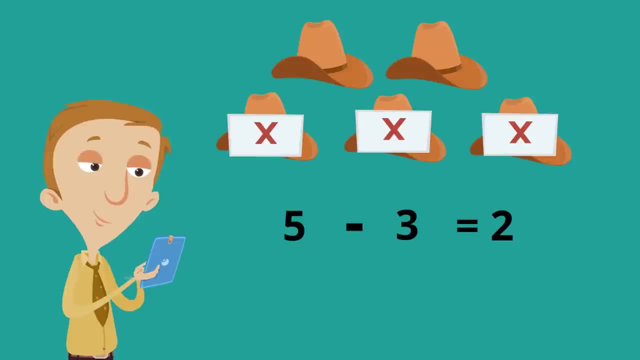 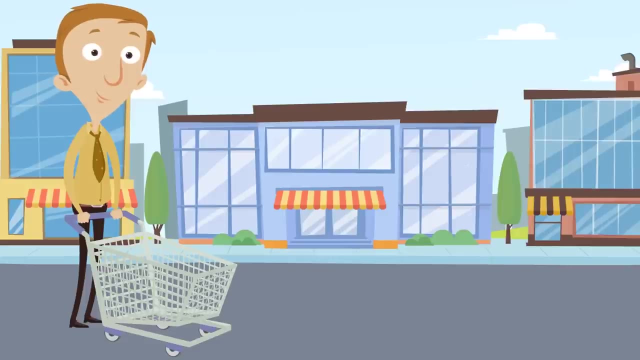 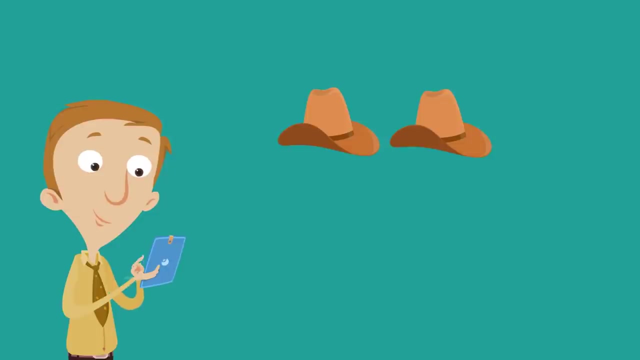 And five minus three leaves you with two. Now I have just two hats. We love subtraction. I mean subtraction is when you take numbers away. And why am I in the middle of the road with a shopping cart? So I have my two hats and that's fun, because then the hat has a friend and they're like: 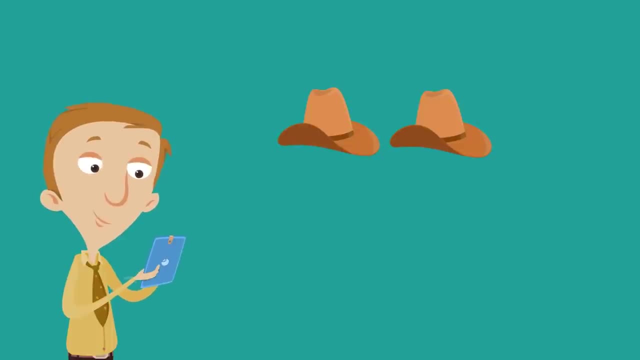 buddies and they're like a pair of friends. And then Chomsky came by and I said: oh, I'm going to have to do subtraction again, I'm going to have to subtract again. Oh, Chomsky, you know that Choms, he came by. 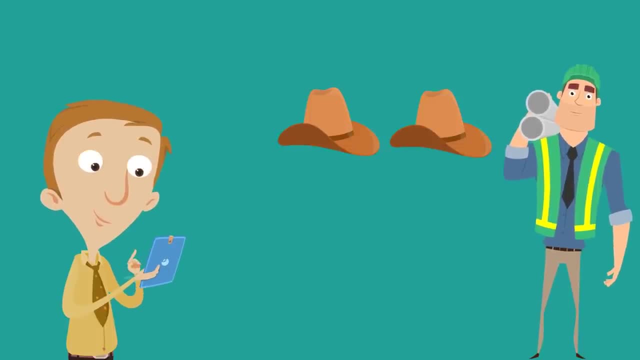 I said I'm going to have to subtract again, I'm going to have to subtract one more time. So I have two hats Minus one, Two minus one. So we subtract that one, We take that one away, And how many hats are left? 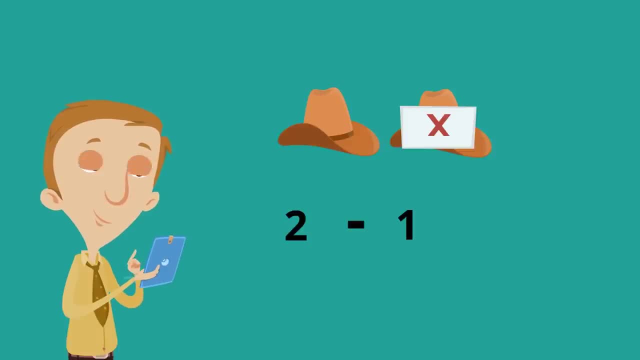 What is two minus one? Yep, Two minus one equals one. There's only one hat left, Which is fine. I mean, you know, I can only wear one hat at a time, and it was the same exact hat. I think about it. 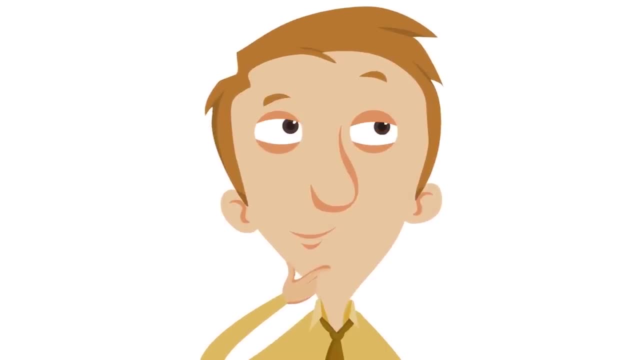 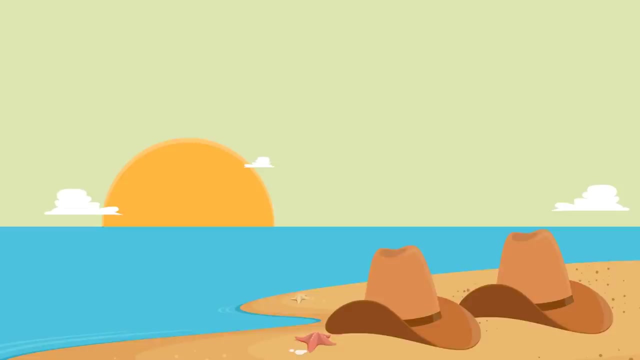 Subtraction has been good to me. It's good Subtraction is taking numbers away. Sometimes I do wonder what would have happened if I didn't give that hat away. If Hattie still had his friend, they could have gone to the beach together. 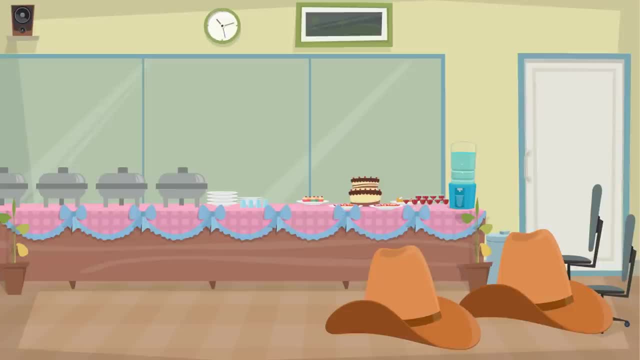 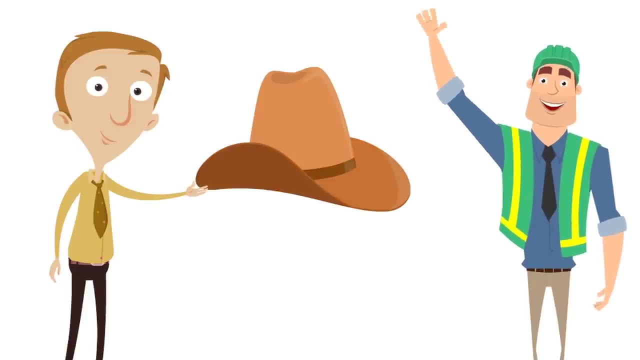 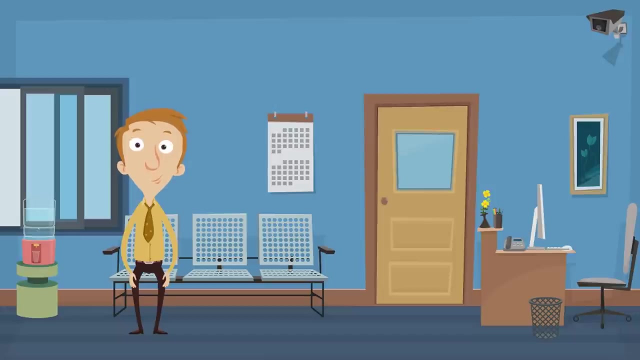 They could have gone to birthday parties, But actually the hat had a better purpose: To make a friend happy. So in this waiting room all I gotta say is: thanks, Subtraction, You are pretty awesome. Thanks for hanging out with us.